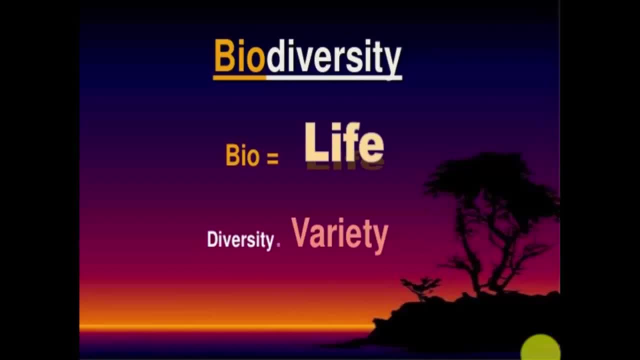 it means the plants, the animals, you know everything that is available in an environment. When somebody says biodiversity, we are actually saying biodiversity. Now, what biodiversity refers to is the very structure of the ecosystem, in, in all respect, right. so biodiversity for any ecosystem, for any environment, is very important. 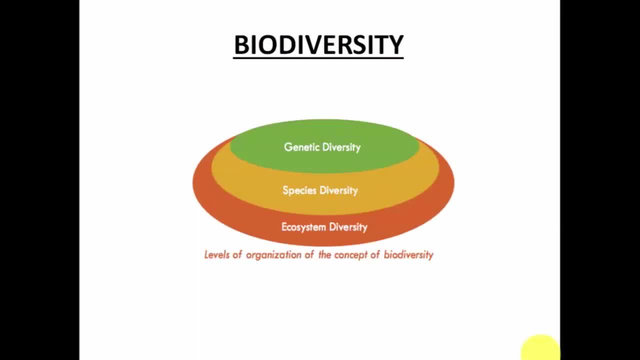 so now, when i say biodiversity, first thing what i have is the genetic diversity. that means genetically we will have in an environment variety of species. a genetic diversity will give rise to species diversity. that is only if the if there is variety in the you know the genetics, then we 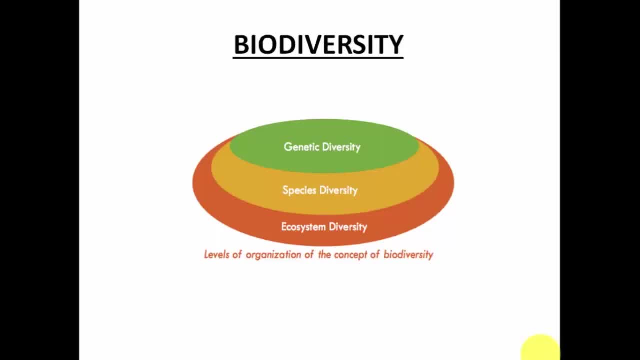 will have variety in the species. we will have a varied species of plants as well as the animals available now. this species diversity will further give rise to an ecosystem diversity that is, diverse ecosystem, different types of ecosystems will be available. so the more the biodiversity, more the ecosystem diversity. right, so that is just a small introduction about. 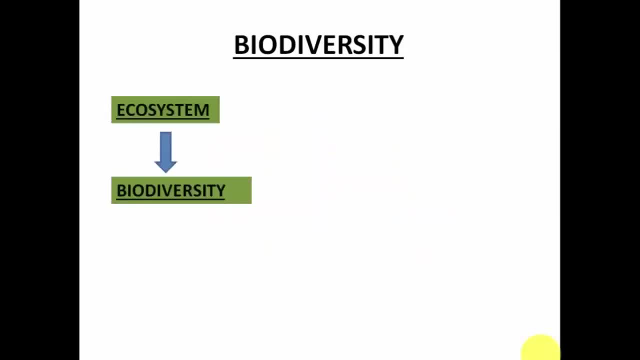 what is biodiversity and why is it very important? let's move ahead. so, as I said, biodiversity is very important for an ecosystem because it measures the health of the ecosystem. our ecosystem will be balanced in all respect, right? if you remember, we spoke about food chain and food web, and by talking about food web, 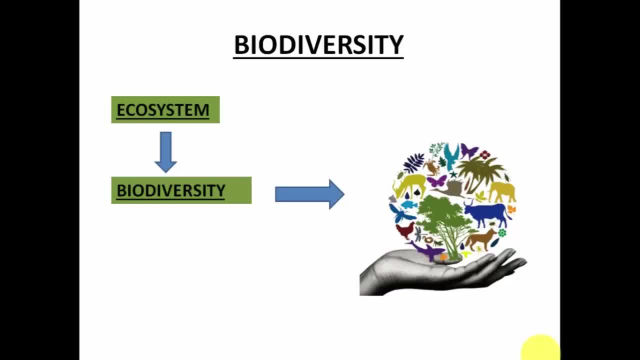 we said that. you know, it is not that for one particular animal he has to eat only one particular plant or one particular other insect or animal, but he has a lot of alternatives available for itself to survive. one animal can eat two other and that particular animal can be eaten by two other animals, or you know? 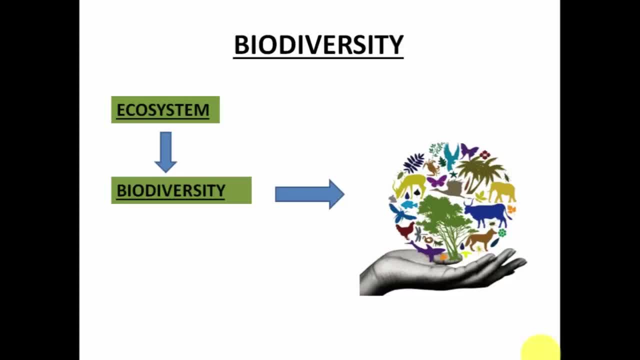 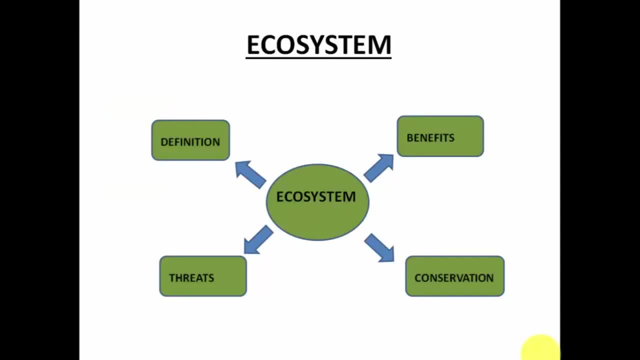 two other consumers. so this is only possible if we have. you know. we said that. you know it is not that for one particular animal, he has a higher degree of biodiversity. now let's move on to discussing the ecosystem. so when we talk about ecosystem, four things very important for 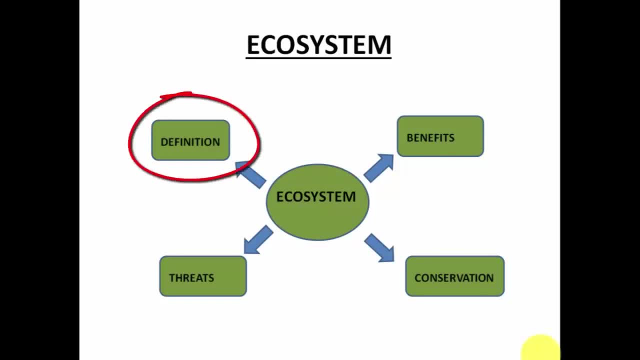 us to learn first is the definition of ecosystem and the normal functions, instructors of ecosystem, which we have already discussed in the previous videos. secondly, the benefits of ecosystem, the threats to the ecosystem and, finally, only if we know about the benefits and the threats of the ecosystem and what the ecosystem means. 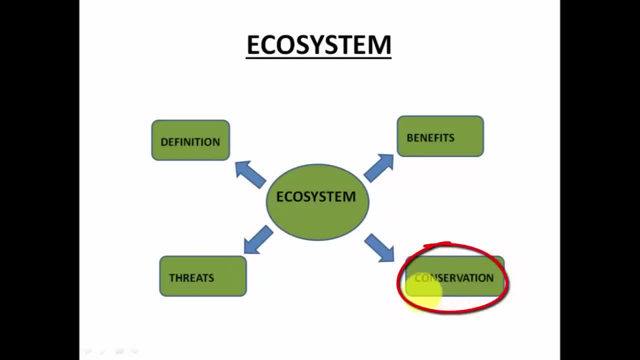 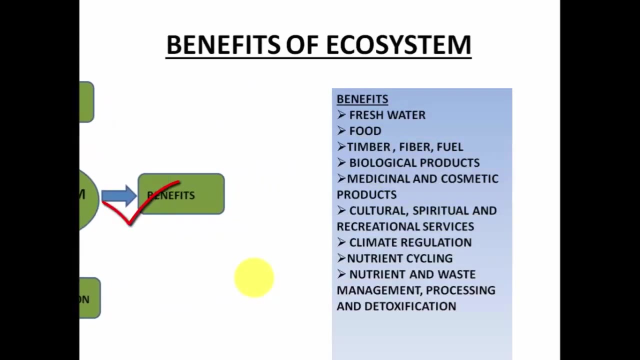 then we will be able to suggest some kind of measures in order to conserve our ecosystem. so in this video we will be talking about the benefits and the threats of the ecosystem. let's talk about the benefits of the ecosystem. the following are the benefits of ecosystem: we have fresh water and food, which is 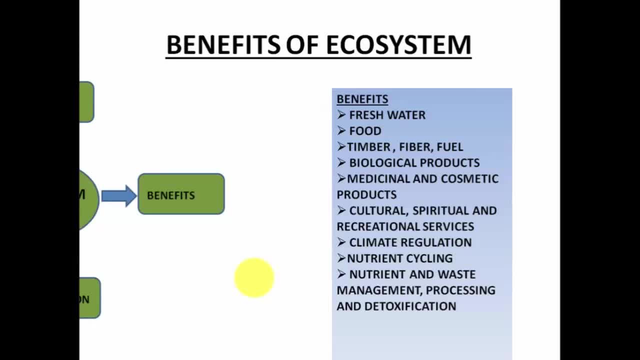 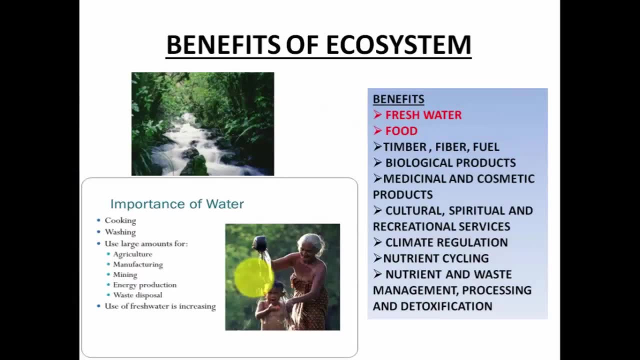 readily available: timber, fiber and fuel, and you know likewise so many different types of deep and river water that grow. so we will just go over them one by one: fresh DVD, dries, cigarettes and other・・ textures and things that should be perhaps considered something like sunlightzne as well as fresh air. so we will just go. 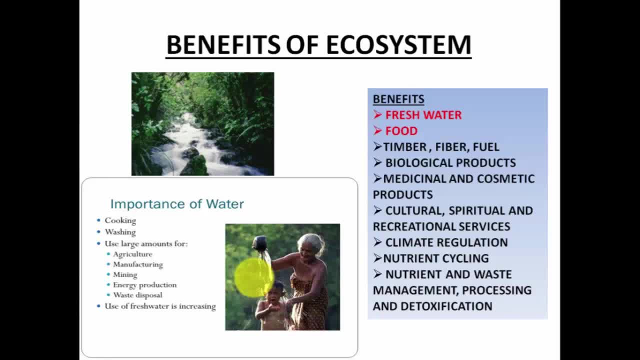 over them one by one, fresh shower water and food. this is self-explanatory. we have for the human population. you know it is. it helps in cooking, it helps us in washing, taking bath. major use of water will be in agriculture, in the manufacturing, in the mining works. also it is used for production of energy. 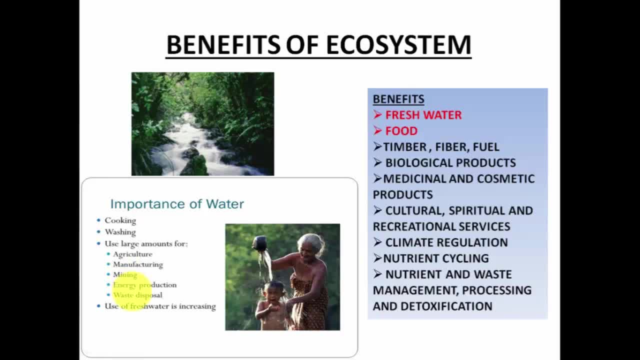 because you know, the turbines are are run with the help of the water and this moving water gives us electricity right. only if we conserve the water resource, if we keep them non polluted, then only the ecosystem can be conserved right. ecosystem gives us food that we eat. it gives us variety of fruits and 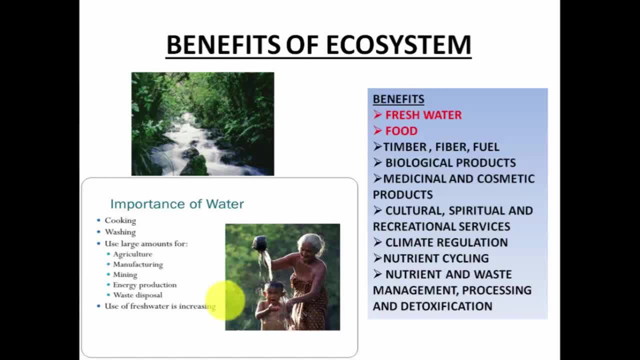 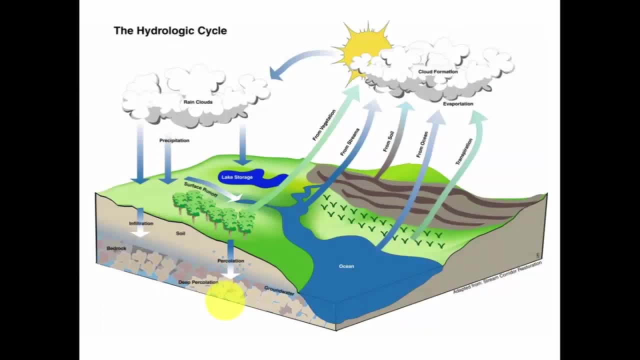 vegetables and cereals available, and this is available to us through agriculture. that is why ecosystem is very important. so water and food are directly available to us with the help of ecosystem. so let's move ahead. how is the water available to us? this is hydrologic a cycle. what happens is the. 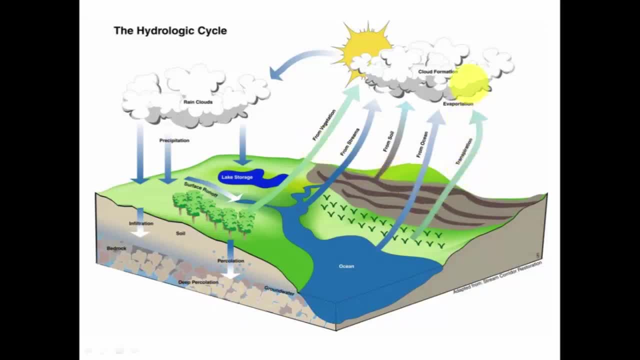 many sources. the water gets evaporated, it gets condensed and this condensation after condensation, again the precipitation takes place, it will, they become the rain clouds and again in the form of rain, the water is again available to these primary producers, and the cycle continues like that. so this is. 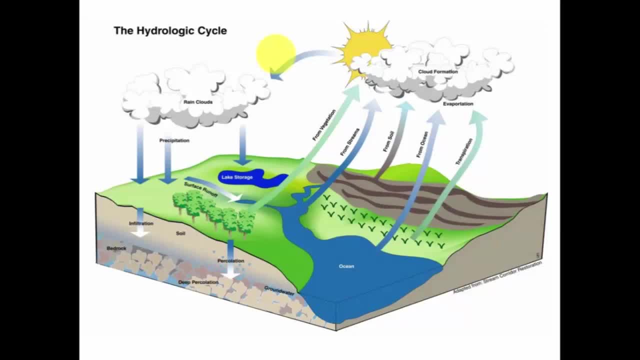 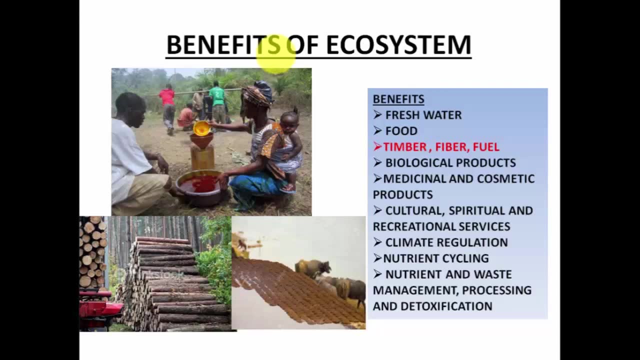 the hydrological cycle and this is the cycle of water and the cycle continues like that. so this is the hydrological cycle and this is the basically how the water is available to us. other benefits are availability of timber fuel and fiber, because, you know, we have a lot of trees available, so the 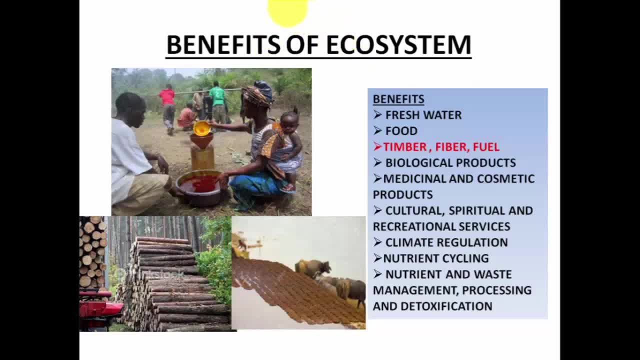 timber is available. we have the cow dung, which is available. so this cow dung is majorly used in the rural areas by the people over there in order to cook their food. of course, it has a lot of health hazards, but then this becomes the primary source for them to cook their food. 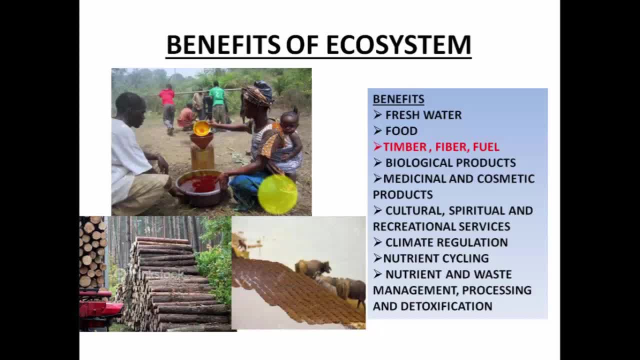 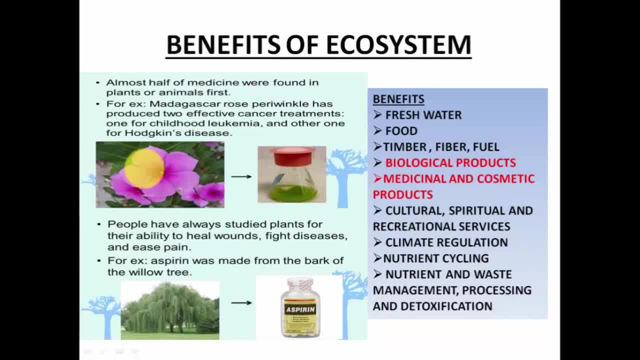 ecosystem gives us a lot of raw material for us to, you know, to use. next is the biological products and other medicinal and cosmetic products are available. you know most of the medicines which are important. medicines are a byproduct of. you know a lot of flowers. they are available because 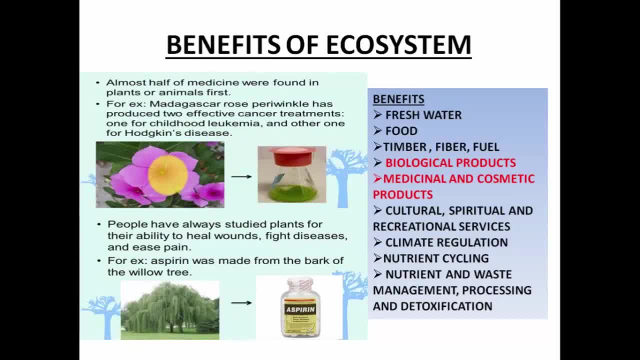 of flowers, for example the Madagascar rose, or, you know, perincle, has produced two effective cancer treatments. one is for the childhood leukemia and the other one is for the Hodgkin's disease. so this flower you must have seen, very, very common flower in your surroundings, also this medicine. 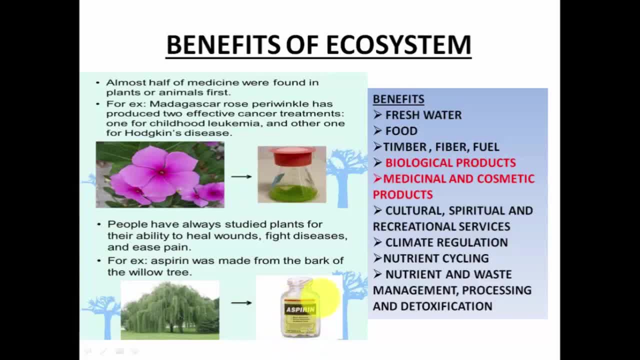 which is known as aspirin. it is also available because, you know, from the bark of this willow tree. so, likewise, most of the trees, most of the plants, they give us a lot of medicinal products which are very important and they are very important for us to use. next is the biological products. 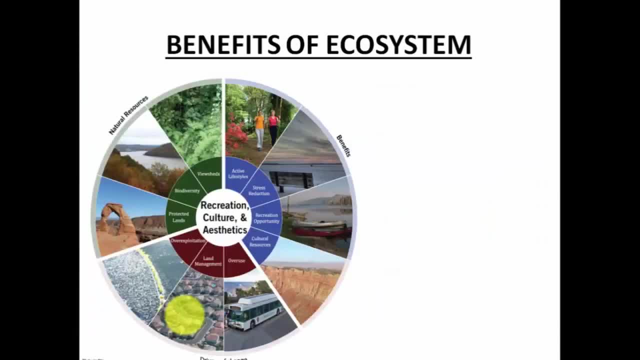 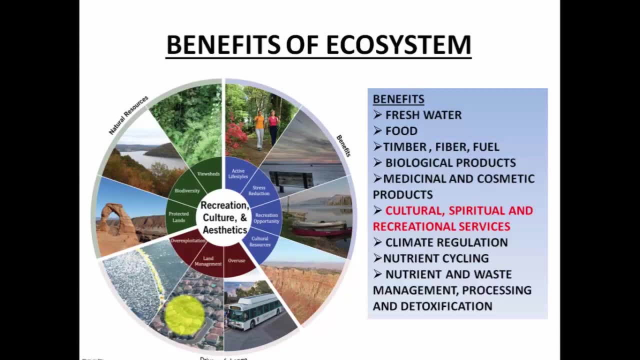 being used in, you know, today's world. next is, uh, the cultural, spiritual and recreational services. these services are also directly and indirectly available to us because of ecosystem. these also come under benefits. these are also benefits of ecosystem, of course. like you know, we have an active lifestyle. we would like to exercise every day in a, in a very clean and a very healthy and. 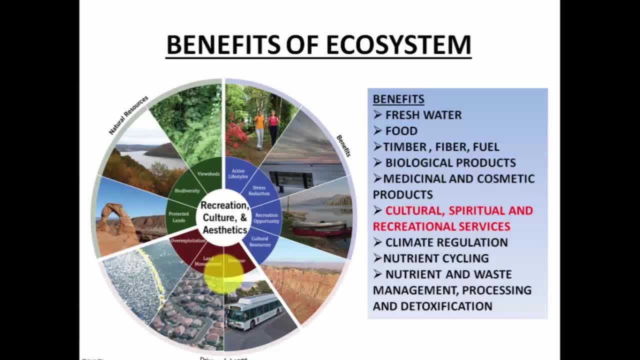 green environment so that environment is available, because we have a balanced ecosystem right. so it gives us a very active lifestyle. also, it is a great stress buster. we have places which we like to visit and, you know, relax, so this helps in reducing the stress. other recreational opportunities. 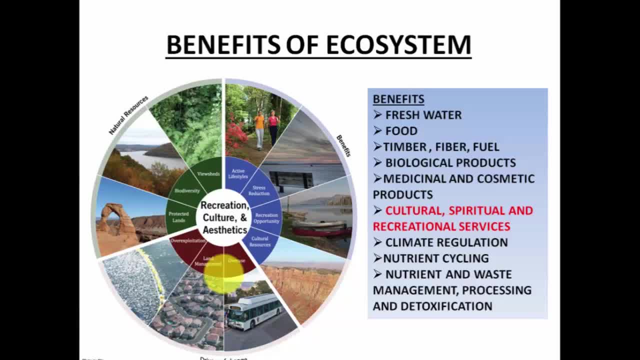 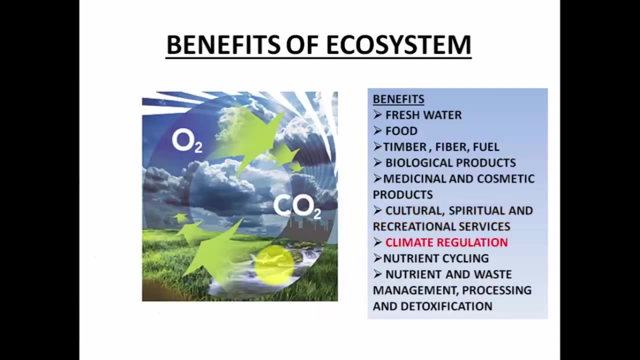 are available, and that is all because of the ecosystems. we have beautiful greenery around us, diversity around us, so all these things are available to us because of ecosystem. that's why we say that ecosystem provides us with cultural, spiritual and recreation services. okay, next is climate regulation. this regulation of climate takes place in many different ways. for example, 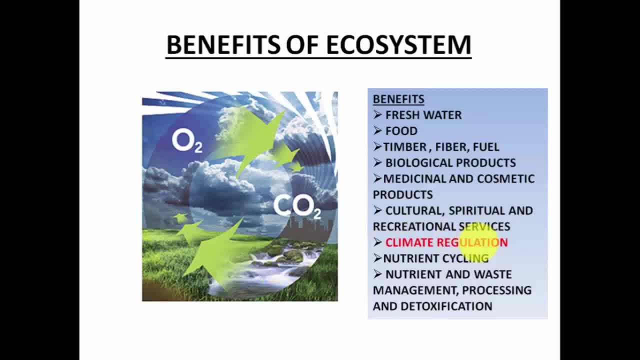 you know, there is, uh, the next point, if you see the nutrient cycling here. so all these are interrelated. only if there is proper cycling in the environment, uh, proper water cycling in the environment, and then nutrient and water, if they keep properly cycling in the environment, then this regulates our climate. you know our. 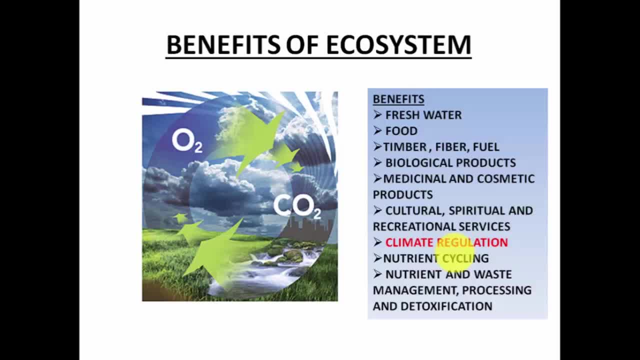 climate is maintained properly. for example, let's say, if we do not have a lot of trees, then there won't be any more rains, right, then, more the number of trees, the more rains will we have, right? so why is that so? because you know the trees: they take in the carbon dioxide, they give out oxygen, they, they make the environment. 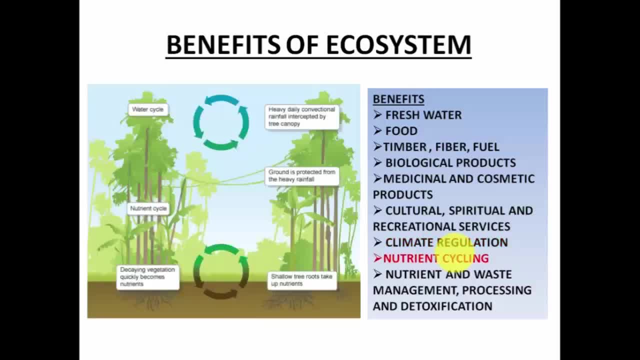 you know, oxygen rich environment. okay, now the nutrient cycling. what do you mean by nutrient cycling? the same nutrients are being recycled again and again. they are being used and they again come back to the soil and then again used by the primary producers. so, for example, you can see on the left we have, on the top we have the water cycle. what 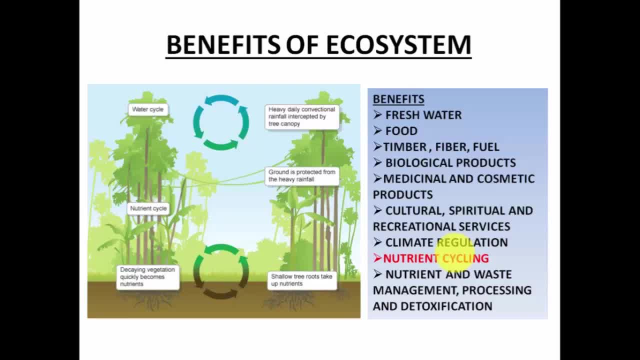 how does a water cycle takes place in the environment? first of all, the trees. they take in the water from the soil. they produce food with the help of a process known as photosynthesis. again, the same water gets evaporated, it goes up and then it become, you know, rain. 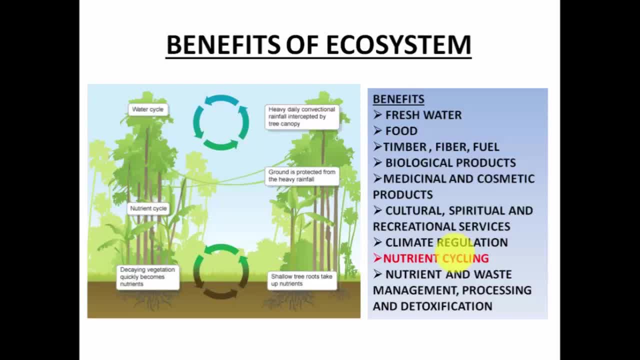 clouds. the rain clouds again precipitates and give rainfall. the water is available to the soil and from there it gets recycled. so that that's how the water is recycled. similarly, even nutrients are recycled. how is the nutrient recycle? first is we have the green leaves, will then decay, and again those nutrients are available in the 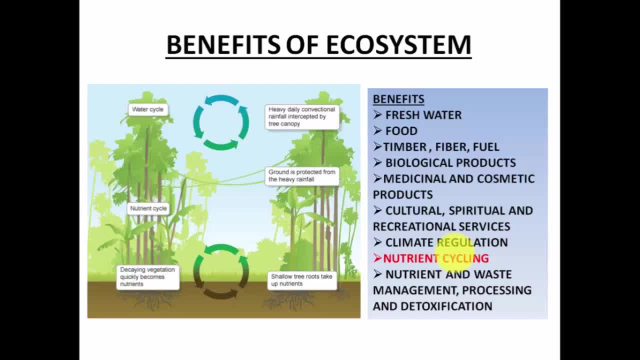 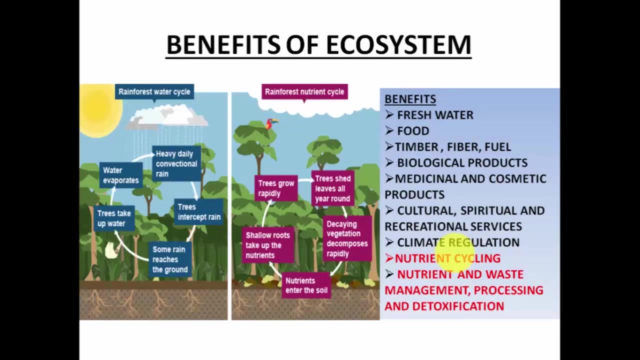 soil, the nutrients are again absorbed by the green plants in order to again make their food. so that is how the nutrient cycling will take place. so it is water and the nutrient cycling both taking place together. this helps in regulating our climate. okay, so the nutrient cycle. again one more time i have shown: on the left is the water cycle and on the right is the nutrient. 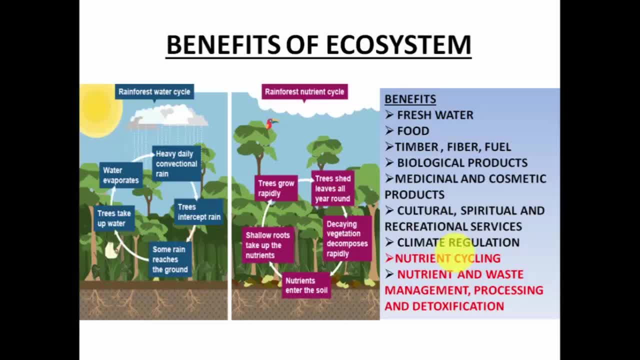 cycle, right? so, because these two cycles are happening all the times- and this also helps in, you know, waste management and processing and detoxification. because, uh, what is detoxification? you know they've taken the plants, taken some of the like co2, so these gases are absorbed and they 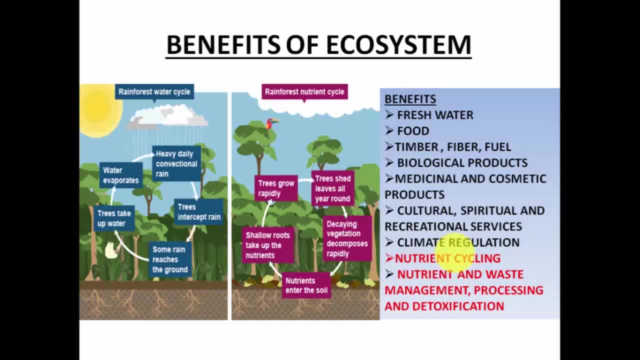 take out the gases which are healthy for us, for example the oxygen, so they basically help in detoxification. right, the waste management. nothing goes waste in an ecosystem. things die, they decay. the nutrients are again absorbed in the soil and from the soil they are again taken up. they are absorbed by 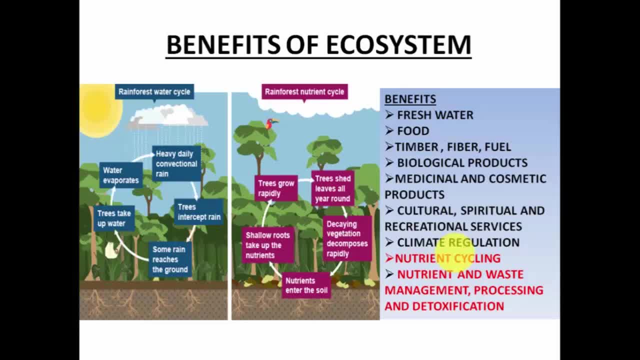 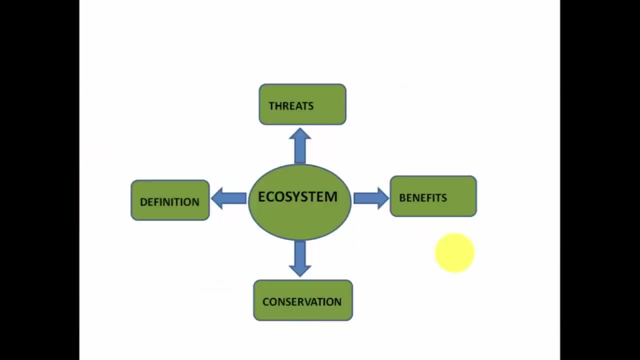 the plants in order to produce their food. so nothing goes waste as far as an ecosystem is concerned, be it, you know, green plants or the animals, everything is recycled, so there is a proper waste management process that is happening in the ecosystem all the time, right? so these are the major benefits of ecosystem. now let's move on to discussing the threats. 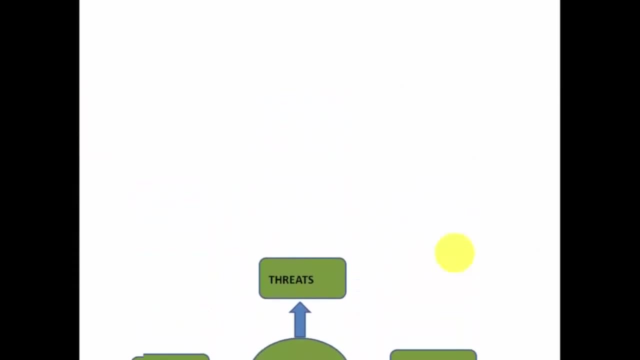 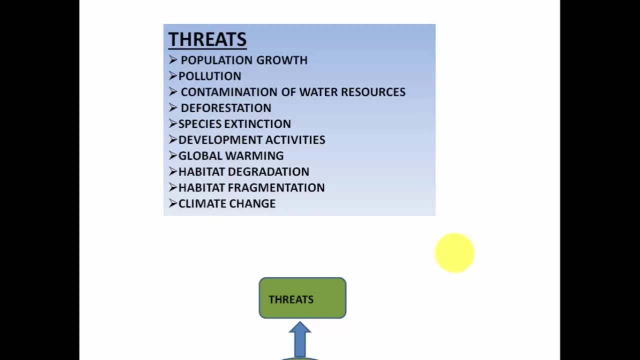 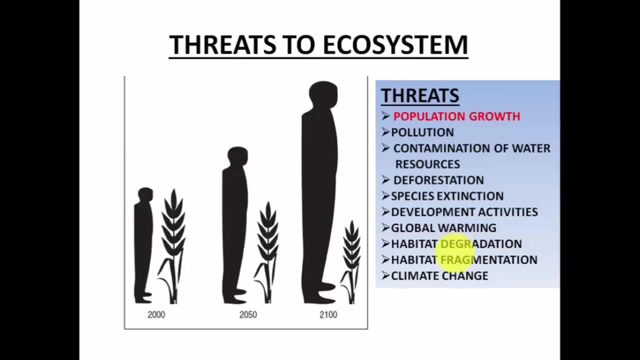 that are available to the ecosystem right. so the major threats are basically the population growth. this is the the first and the foremost threat and because of this population growth, the the rest of the threats that we see on the screen rest of the threats will follow automatically, but the major threat is the population growth right. so let's say, if i have 100 people in 2000, 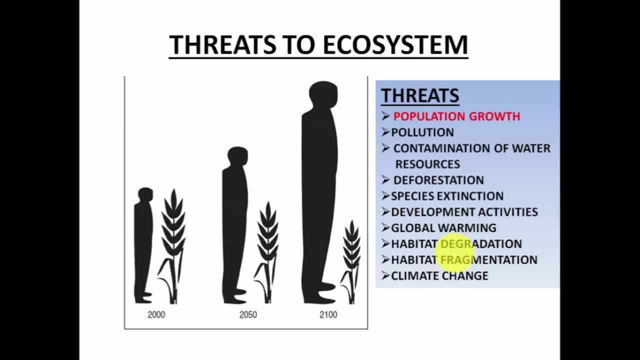 and then in 2050, let's say, it is expected to become, you know, thousand people. so for thousand people, the available resources, the available food, the available water will be less and the population is more. so again in 2100, you see, the population is rising at the same rate, whereas the 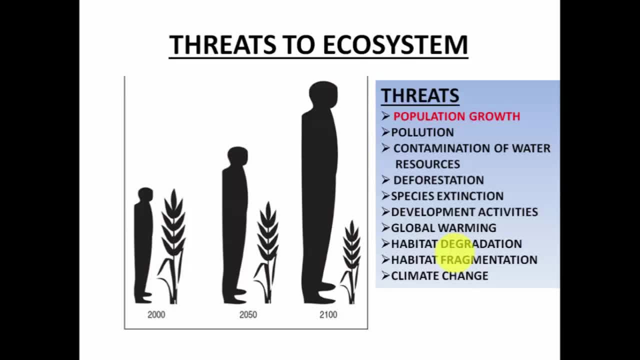 amount of food that is available will be even less so. this shows that, as a population is growing, the amount of food that is available for each and every individual will become will slowly be reducing, right. so that is why i said when the when there is a growth in the population, if the 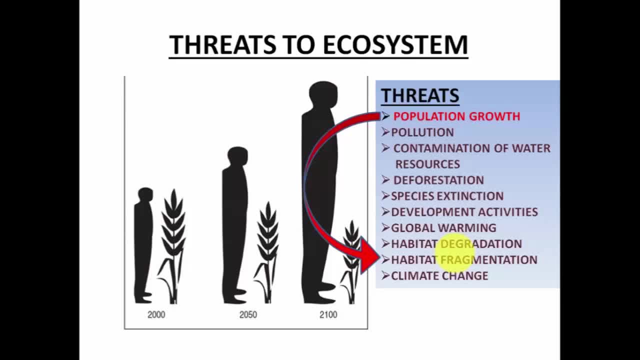 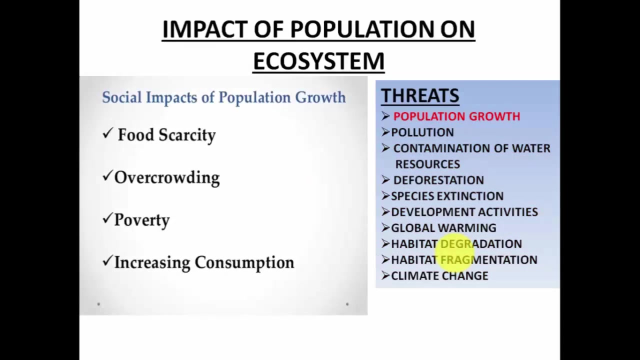 population continues to grow like this. the rest of the threats, that is, the pollution, the contamination of water resources, the deforestation, the species extinction, development activities, global warming, habitat degradation, defragmentation and climate change. so all these threats will automatically follow again when the population increases. firstly, as we discussed, the food scarcity. 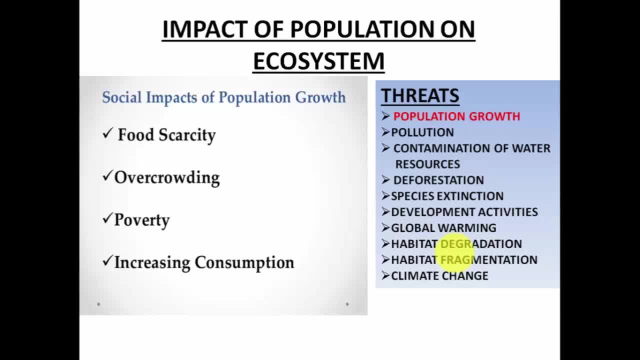 will follow. there will be overcrowding because of the lack of water. so this is a very important: population is increasing. they'll be overcrowding in a particular area because the area available on the earth is the same, but when the people are increasing, when there's a growth in the population, 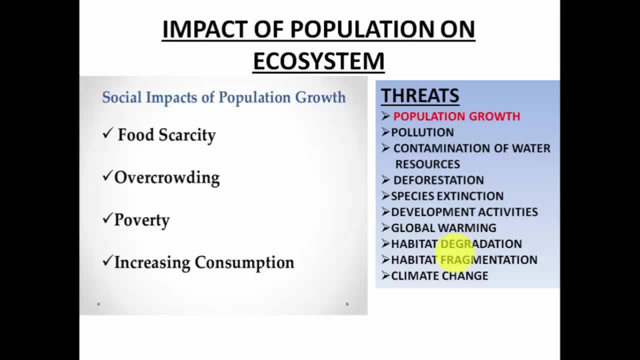 then they will be overcrowding. people will have less place to stay. poverty will increase because the resources are the same, the food is the same, you know, the jobs are only that many, so the poverty will increase. last is increasing consumption. that is, if the population is increasing, then the 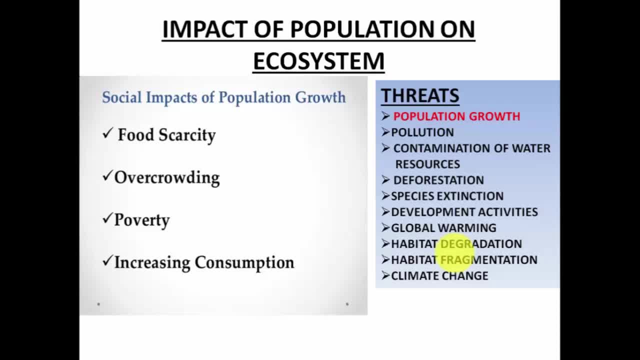 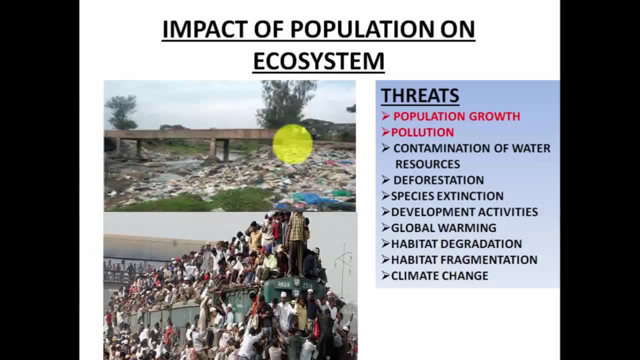 consumption will be more consumption of water, food resources, whatever you can think of. so what is important here is that the population has to be controlled. so now, coming on to pollution, it is but obvious that if there is population, the growth of population continues like this, then the pollution will also continue in the same way. 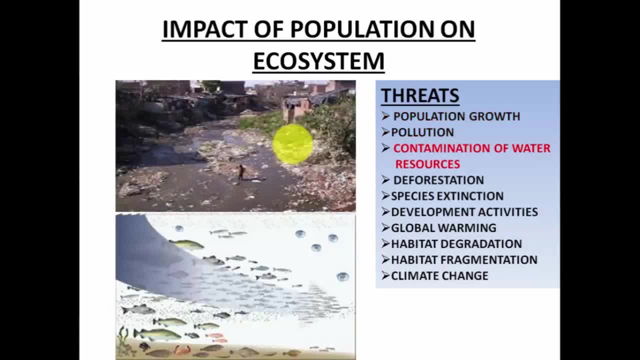 so the more the population, the more the pollution. what is the consequence of this thing? if the water resources get polluted, the species that are staying in that water resource will get affected, their health will get affected and in turn, you know, humans are eating those fishes. we are the ones we eat fish, we eat lot. 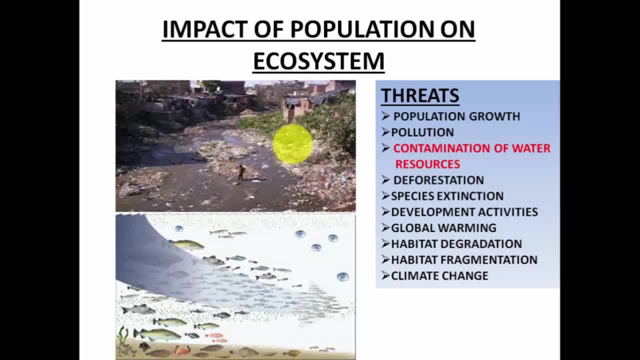 of other seafood. so in turn, what happens is such a water resource will also indirectly be affecting even our health. what is important here is to avoid this kind of pollution, to avoid contamination of the water resources, because, you know, if we avoid this contamination then this is a way we can keep our ecosystem. 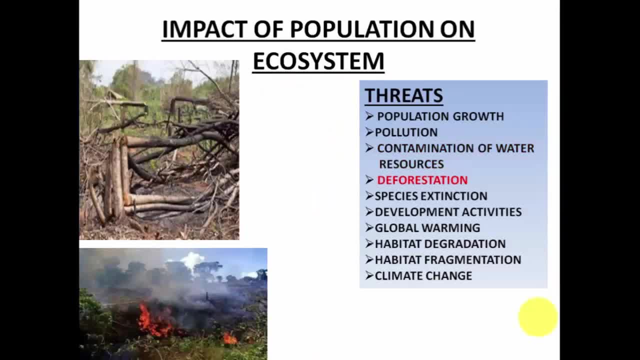 healthy. next is deforestation. because of the growth in the population, humans wants to reach out at every location. they wants to, you know, uh, build up new industries, they want to build up new localities. so, and how do they do that? they are cutting a lot of trees, they're burning a lot of jungles, they're cleaning all the 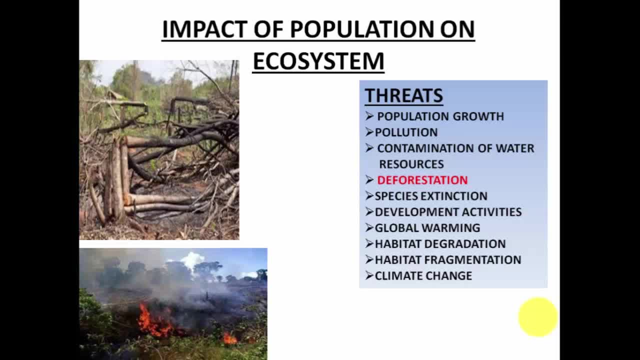 jungles. so this kind of pollution is going to be affecting the ecosystem and this kind of deforestation is affecting the ecosystem also because you know, if the deforestation takes place then the wildlife that are staying in that jungle or in that area, in that habitat, gets. 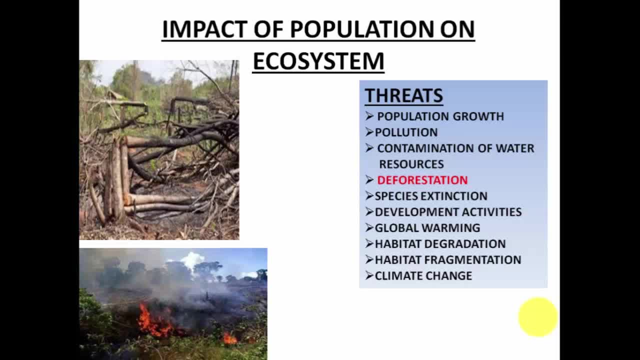 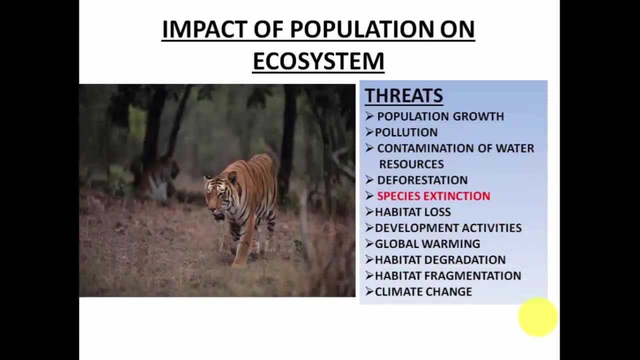 relocated, gets disturbed. so deforestation is a major cause for the wildlife which is getting disturbed. so the major impact of growth of population on the ecosystem is deforestation. deforestation leads to species extinction because the jungles have been burned, the jungles have been cleaned, a lot of deforestation taking place. 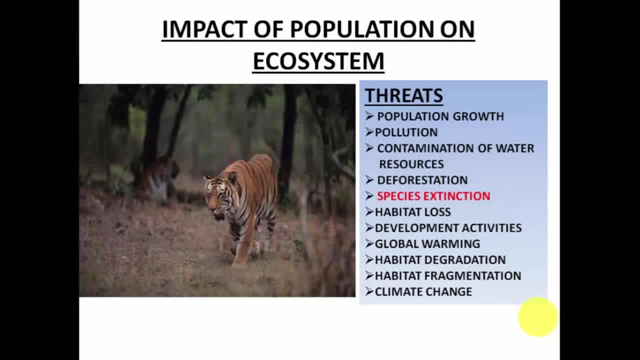 so, ultimately, the there are a lot of species which are extinct today- a lot of birds and the tigers we keep hearing. so these species are getting extinct and this is not a healthy state of any ecosystem. so we need to keep the species intact, right and because keeping them intact will only lead to higher 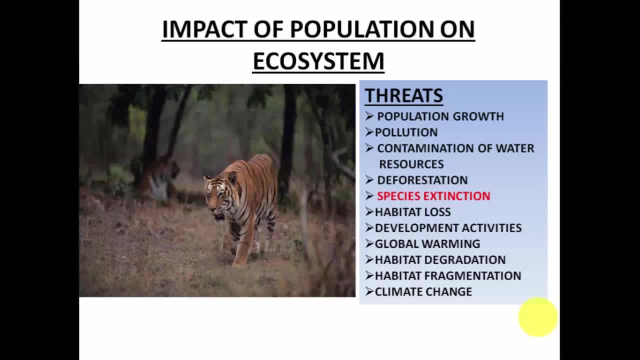 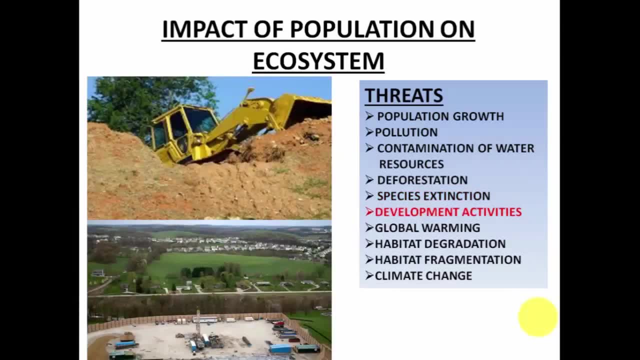 biodiversity right. so major impact of growth of population is one is species extinction. next is development activities. because of growth in the population, there are a lot of development activities, a lot of construction that is taking place. that is exactly the reason why a lot of forests have been burnt and clean deforestation is taking. 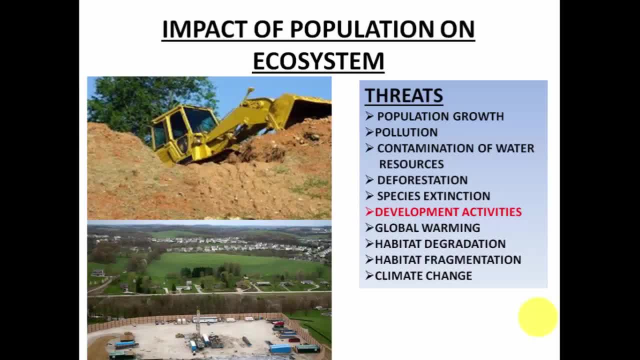 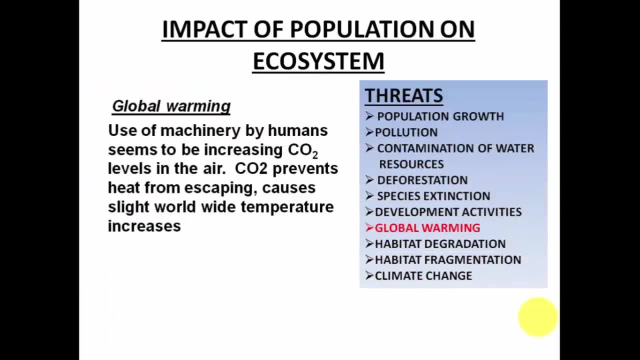 place. such development activities again results in, you know, imbalance in the ecosystem. now let's move on to global warming. global warming is also one of the major factor which disturbs the ecosystem, and global warning is also a result of the growth of population. use of machinery by humans seems to be increasing. 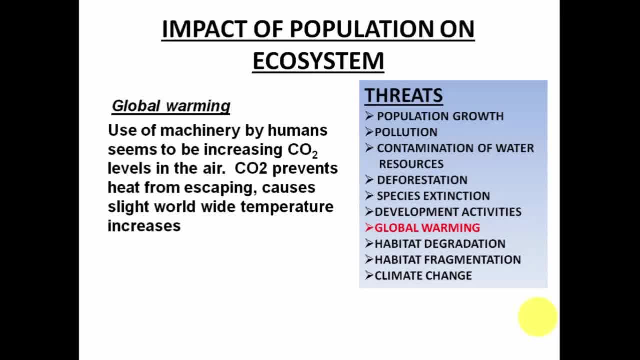 uh day by day and this increases the amount of co2 that is available in the air and this carbon dioxide prevents the heat which is escaping from the surface of the earth and ultimately, what happens is the climate changes because co2 remains inside our, inside the environment. here. 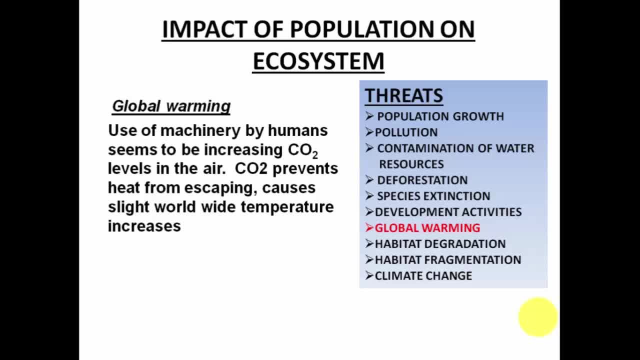 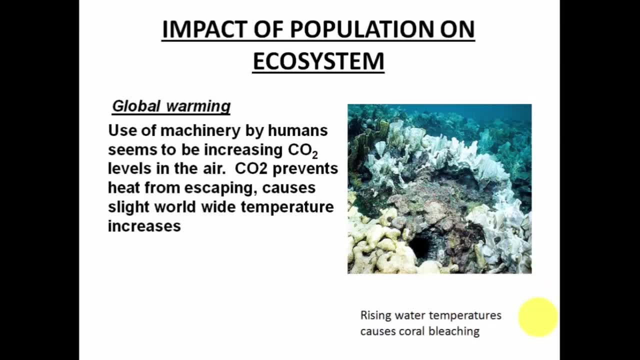 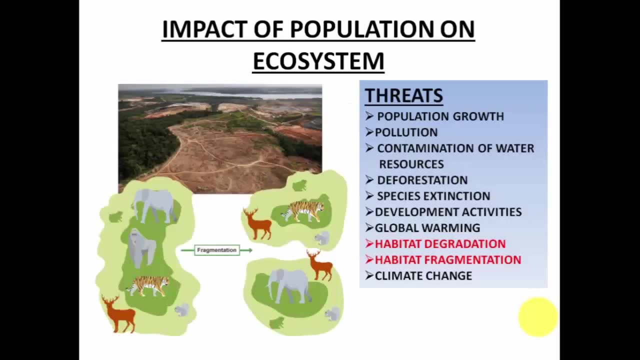 on the earth. so this increases the temperature of the earth and this is known as global warming. what is the effect of global warming? you can see on the right: because of the rise in water temperature, this kind of coral bleaching is taking place. next is habitat degradation and 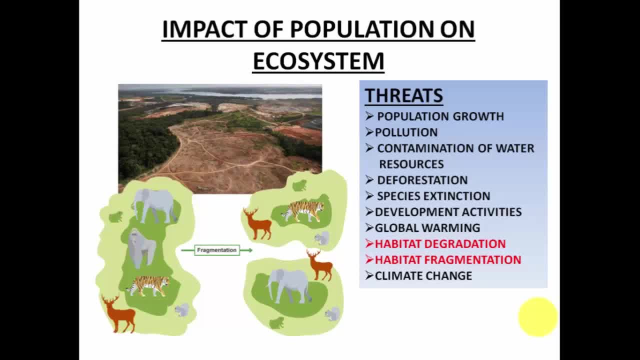 habitat fragmentation. uh, they are the result of the growth in the observation of coral bleaching, which leads to rising vegetation. on the left, you can see, the habitat is a huge habitat, big without any fragmentation, whereas on the right, after the fragmentation takes place, the wildlife is separated. and why this fragmentation? 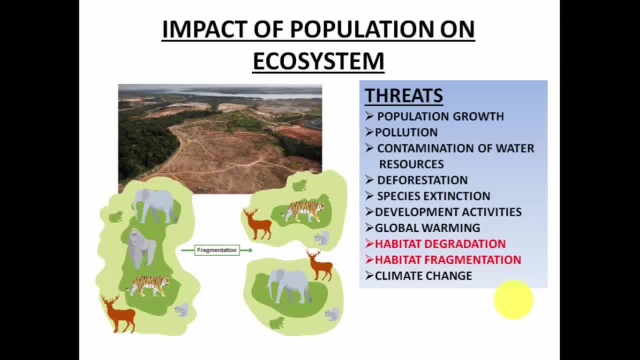 why do? what do you think is the reason for this fragmentation? definitely human beings. we want to make a lot of roads or some kind of activity must have taken place and that's why the fragmentation is taking place. and because of fragmentation, the species are separate. this these wildlife will have to relocate themselves. this disturbs the entire ecosystem. 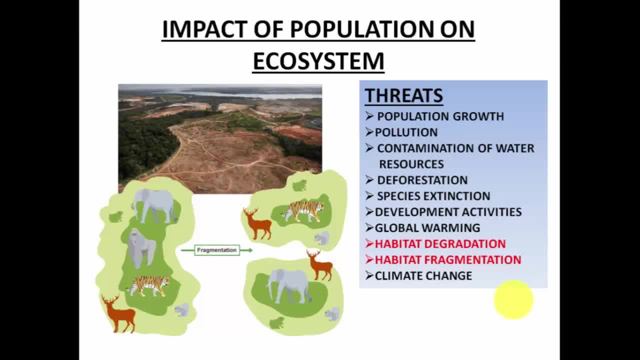 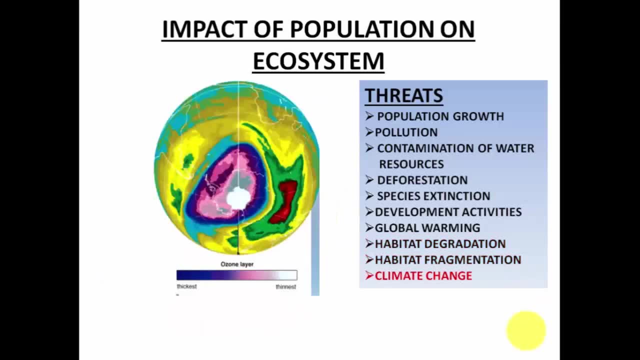 right. so habitat degradation and habitat fragmentation is also a result of growth in the population. so now, when we talk about climate change, one of the major cause of concern is the ozone depletion. the ozone layer is getting depleted. and why is that the ozone layer is getting depleted is because of the chlorofluorocarbons. these, primarily, are found in the 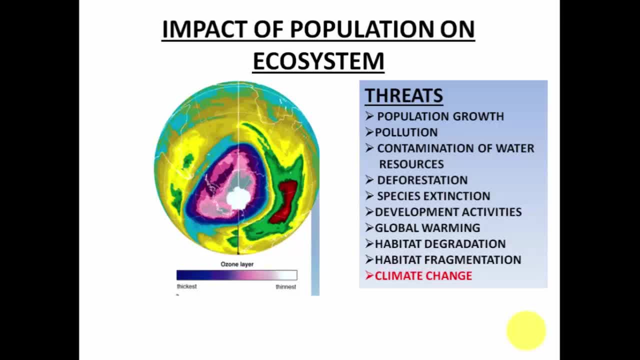 aerosol, spray cans or the refrigerants and they're released in the atmosphere. so what happens is these gases, through several chemical reactions, they cause the ozone molecule to break and that's how the you know they're these. now we see a hole in the ozone layer and the effects of this hole. 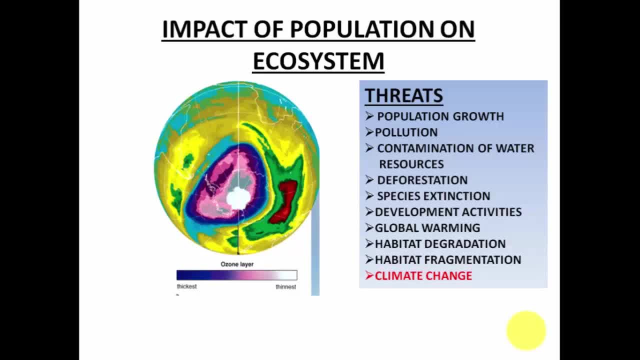 ozone layer is a layer which actually avoids any ultraviolet rays to penetrate inside the surface of the earth, right the environment of the earth. so now, if there's a hole in that ozone layer, the uv rays can very easily pass through the layer and they can reach out to the earth. and 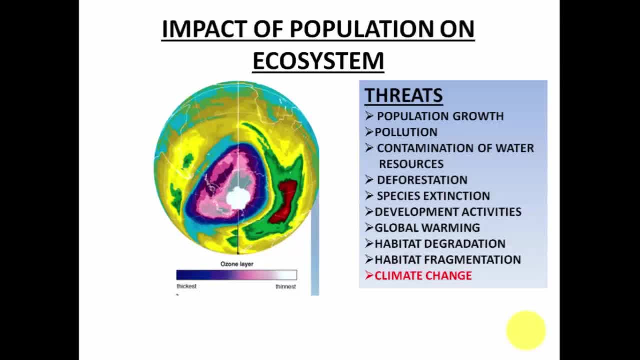 this cause a lot of uh problems, like a lot of disease, like skin disease, because, you know, because of the increasing population, there is a lot of imbalance in the ecosystem and somewhere that imbalance in the ecosystem is has affected the ozone layer also, right, and this is a major cause of concern now that we have talked about the threats to the ecosystem, which is 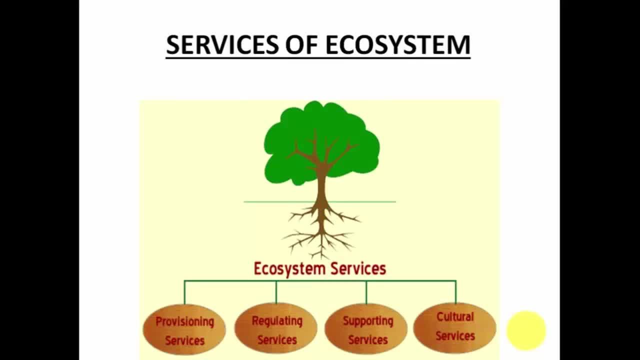 mainly the growth in the population. let us also talk about the services of ecosystem right. so you understand how these services are interrelated to the benefits and how those are integrated to the, to the threats, uh, to the ecosystem. so the ecosystem services are of four types. one is provisioning services, regulating services. 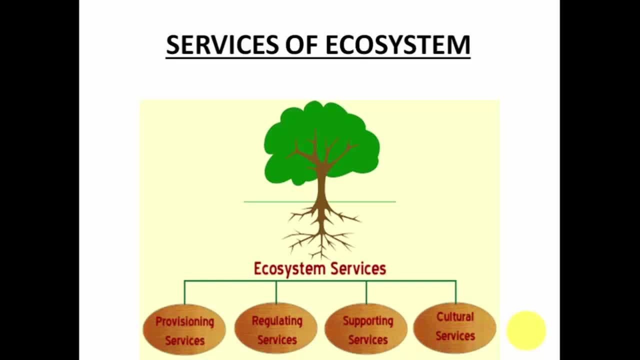 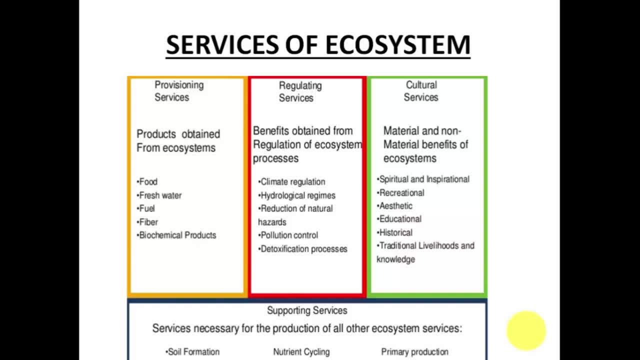 supporting services and cultural services. so let's see what these are. under the provisioning service services, products that are obtained from ecosystem comes in this. so when we talked about the benefits of the ecosystem, we said ecosystem provides us food, ecosystem provides us water. we also talked about some, you know, biochemical products. 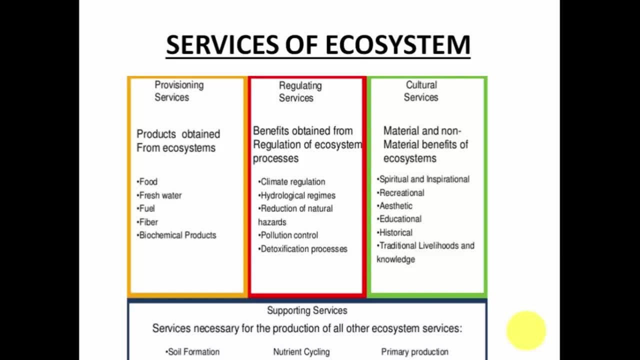 some medicines. we talked about fuel, fiber, timber. so those are the provisions, those are the provisional services that the ecosystem is providing to us. next is regulatory services. these are the benefits that are obtained from regulations of ecosystem processes. for example, we have the climate is regulated, the hydrological regimes, the reduction of the natural hazards. and what are those rough 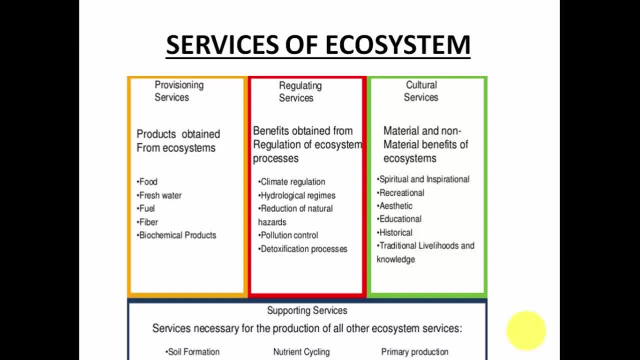 in the natural hazards. we said waste management, you know, detoxification, so all that process, and pollution control, so all that process will come under regulatory services, right? third is the cultural services, so these are the materials and non-material benefits of ecosystem. we talked about a spiritual, then inspirational, creational, recreational, aesthetic, educational, historical. 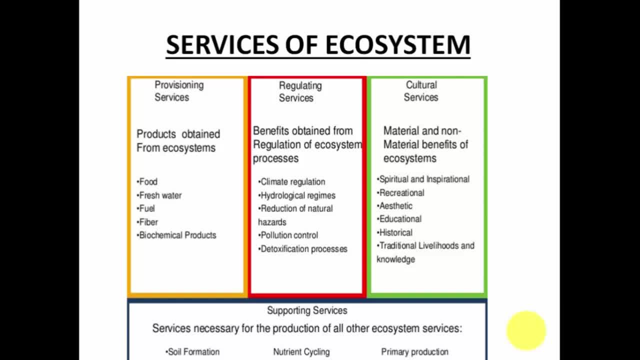 and all these services. so they are the cultural services, so all these services. we talked when, while we were discussing about the benefits of the ecosystem, and now you know to. to just sum it up, i'm just giving you that which all benefits come under which all services. so now we have supporting service. last is a supporting service: services. 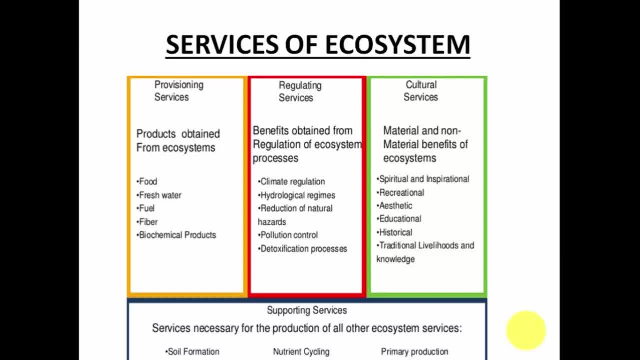 necessary for the production of all the other ecosystem. and what are these primary services that are so important that they regulate even the other ecosystem? First is soil formation. Soil formation is the most important because unless and until the soil formation is taking place, the primary producers will not be able to use it and will not be able 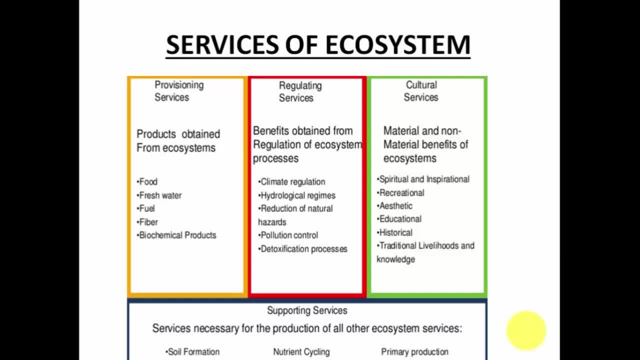 to produce food. So soil formation, nutrient cycle is very important, because that is also that is important to the plants again, and primary production, because primary production has to be there. So soil formation, nutrient cycling and primary production are the three important services that are supporting services, because they end up supporting the neighboring ecosystems. 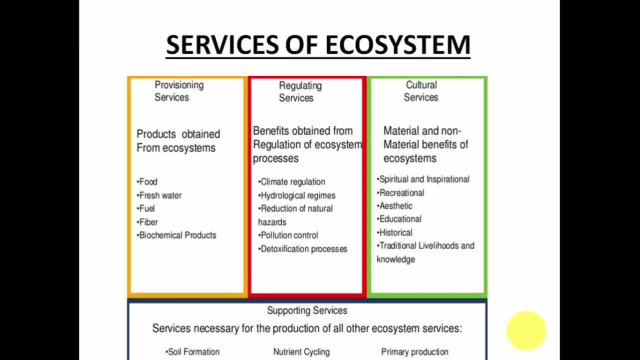 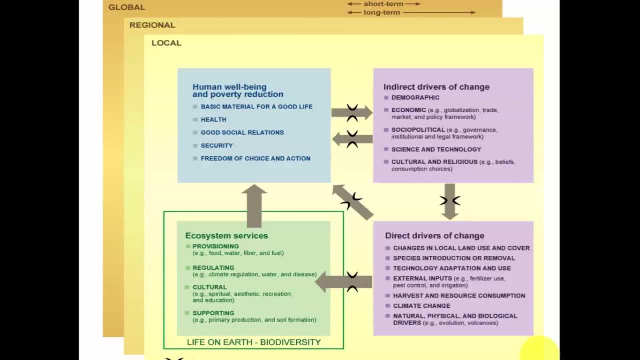 also right. So these are the services of the ecosystem. In another terms, we could call all these services, as you know, benefits of ecosystem. This is what ecosystem provides us with. So now this is a table that will explain to you the relationship between, you know, the human well-being and the ecosystem services and the other direct 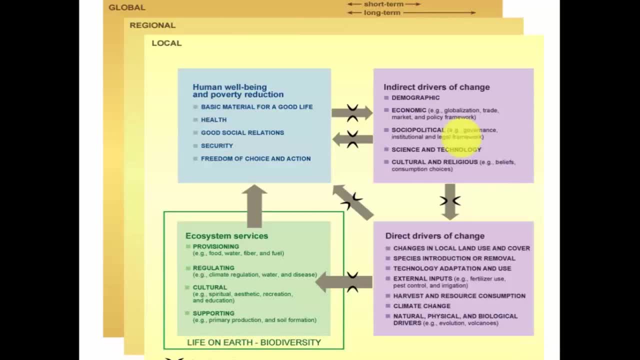 and indirect drivers of change. So the change in drivers that indirectly affect the ecosystem, such as population, then the technology lifestyle, that is, these, I am talking about this box- These are the indirect drivers of the change. They can lead to changes in drivers that directly. 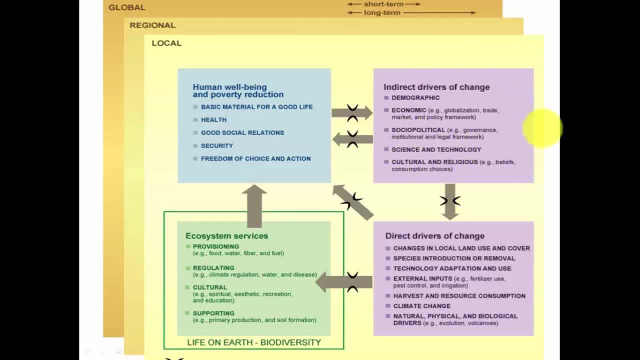 affect the ecosystem. So these are the indirect change which will indirectly affect the ecosystem, for example, science and technology, culture and religious, sociopolitical, economic and demographic. They indirectly affect the ecosystem. But then these changes may lead to some changes which can directly affect the ecosystem, like you know, are changes in local land use and cover. climate change, harvest and resource consumption. why are you levels and you know what kinds of pictures can be sent every겁 тут. like you know changes in local land use and cover climate change, harvest and resource consumption and that does affect our ecosystem And hardcore and neighbour is going to cause the ecosystem to trace your. 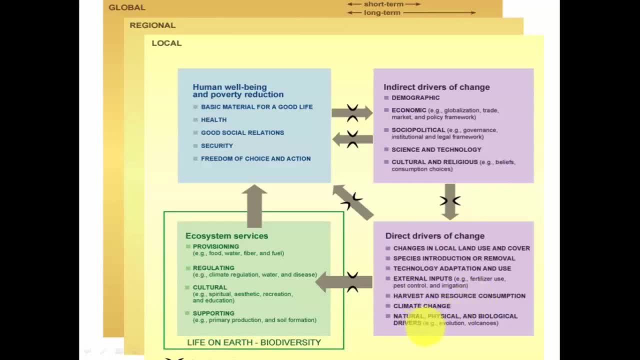 but not the kind structures that are heard in this form. So just a habit will Health, which is your health- natural, physical and biological drivers, so, for example, the volcanoes, evolution- all these drivers can directly affect the ecosystem. and when these drivers directly affect the ecosystem, that means 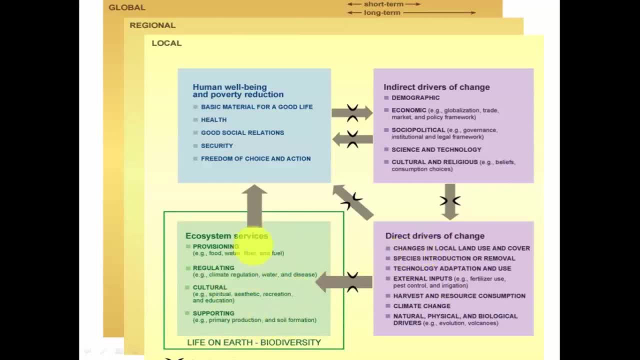 they will affect all these services. if these will change, they will affect this, that is, the provisioning services may be affected. food may not be available, clean water, pure water may not be available. you know, proper regulation of the water and those water cycling or the nutrient cycling may not take place. we may not find a very, very clean and healthy environment for us to enjoy. 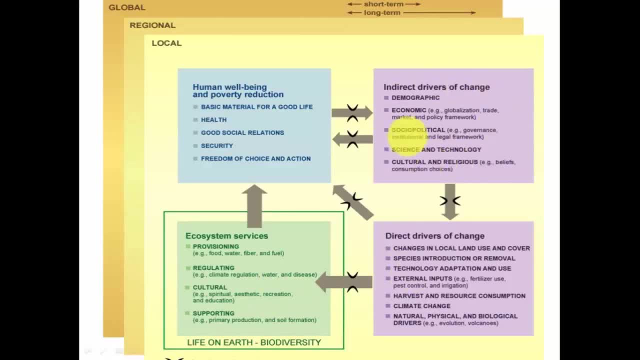 the surroundings. you know. so when indirect drivers change, they in turn change the dummy drivers and these direct driver will affect the ecosystem services. when these ecosystem services are affected, they this in turn affect our well-being, that is, human well-being also. the direct drivers can directly. 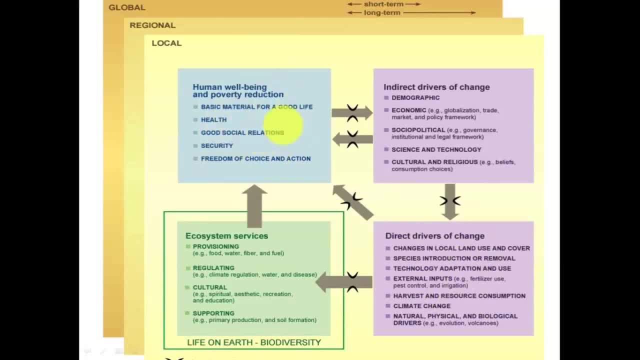 affect human well-being, right. however, all these three- that is, indirect, direct and ecosystem services- can independently affect our human well-being and poverty reduction right. so that's how all these are interconnected. all that we are working towards is to make our life healthy and stress-free. what we have, why are we making the ecosystem a balance and a healthy ecosystem, that is. 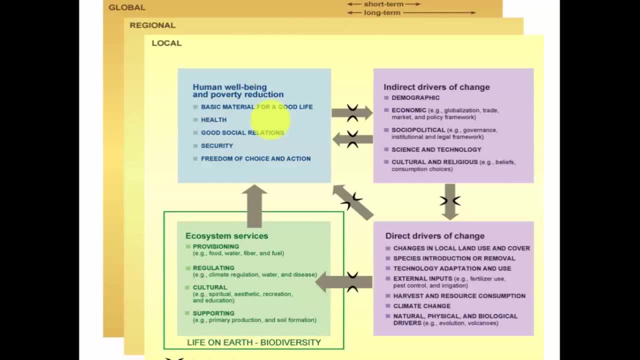 because we want to stay healthy, we want to stay happy and stress-free, and that is why study of ecosystem is so important. okay, so i hope you must have understood the concept here. this applies at the local, regional and even at the global level. also, let's move on to the next one. 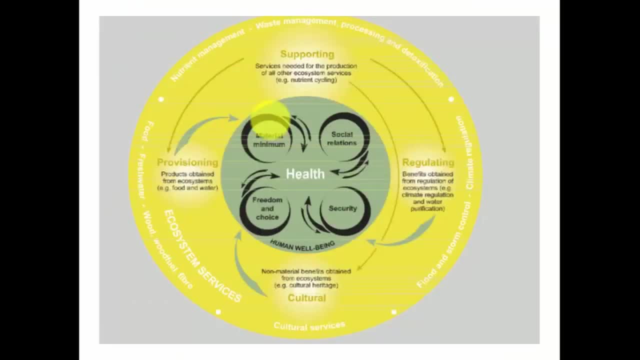 on to this chart again. in this chart you can see health is in the center. that is because. why are we discussing so much about ecosystem? is because we are more concerned about human being, about our health, right, so we consider that the health is the most important. and all these? 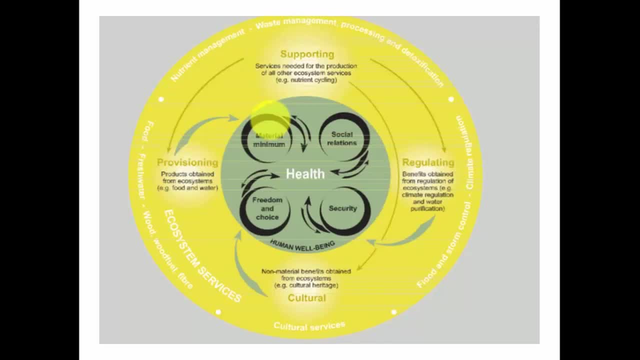 supporting regulatory and cultural and provisioning services are all there just to support the human health, our health right. so health is the one that is will be directly affected. however, there are other small uh things like social relations, security, freedom and choice- here material minimum. so all these four factors can also directly or 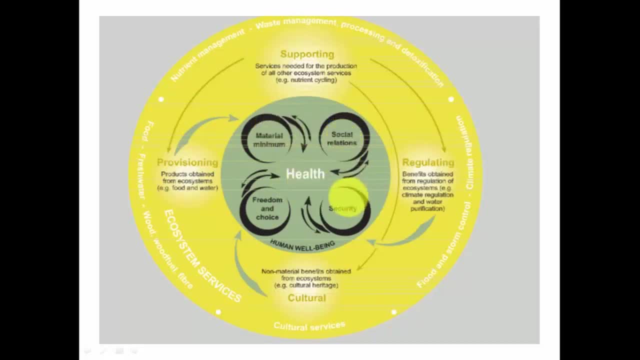 indirectly affect the human health. and these four factors are regulated by the four services that we previously discussed, that is, a supporting service, regulating service, cultural and provisioning service. and how can all these services be regulated? only if we have proper waste management, processing and detoxification process, if we have proper process to regulate the climate. 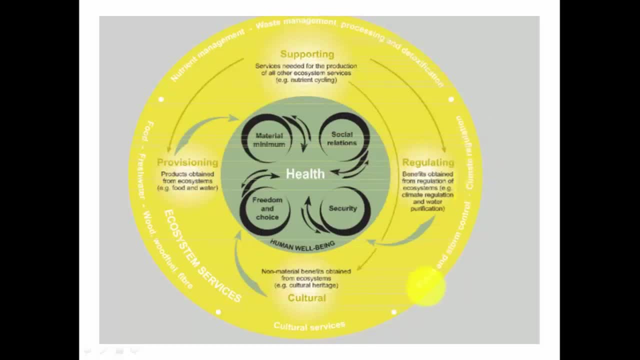 and that will happen when our ecosystem is balanced and healthy, if we have flood and storm control, if we have cultural services, if we have, you know, the fresh food and water and wood, all those fiber that is available, for sure, and flavors, size and filters we should be able to, will be able. to utilize those cleaning soigt Nhou. credibility of the operating infrastructure. therefore manage: if we have proper waste, that's a part of savring processes and detoxification processes. if we havewe have proper process to regulate the climate, and that will happen when our ecosystem is balanced and